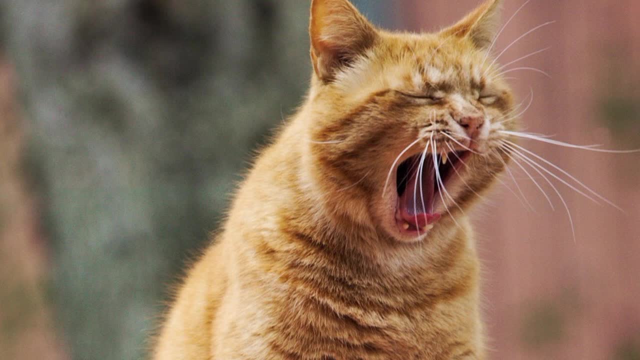 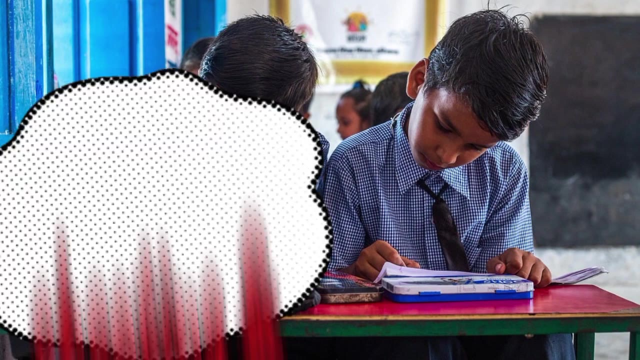 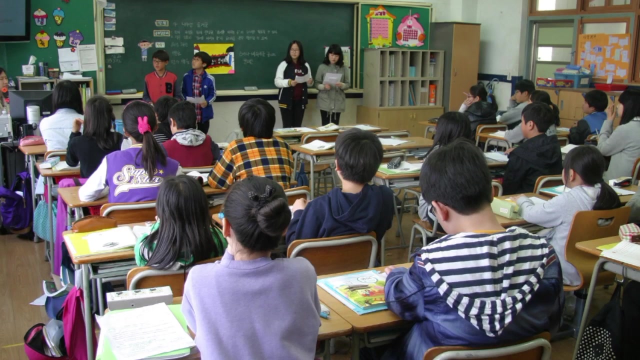 We feel that it's so boring. So the main reason we didn't concentrate: when we are in the class with our friends, we cannot cheat And us can MCQs quite easily. but in the examination hall there is a lot of students and there are students. 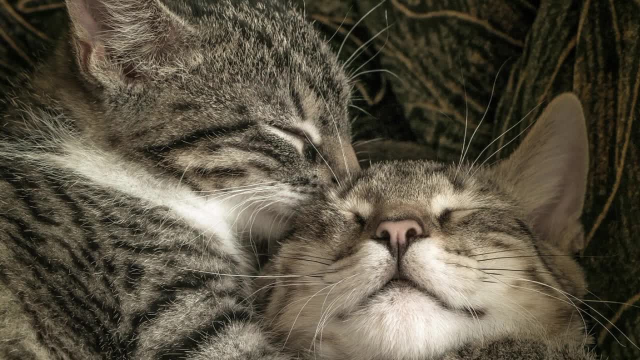 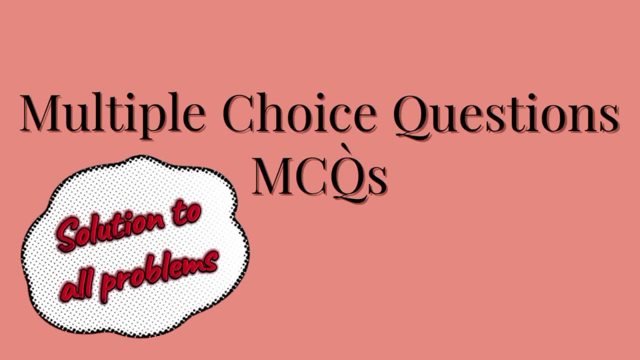 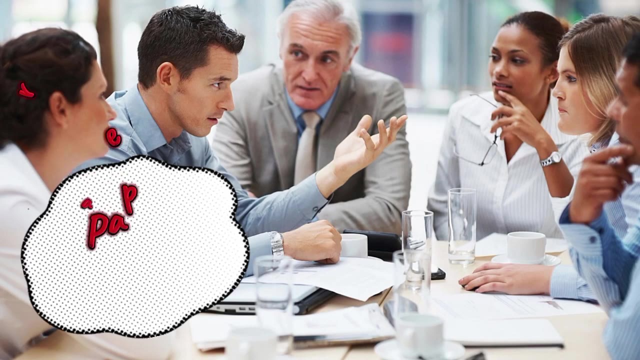 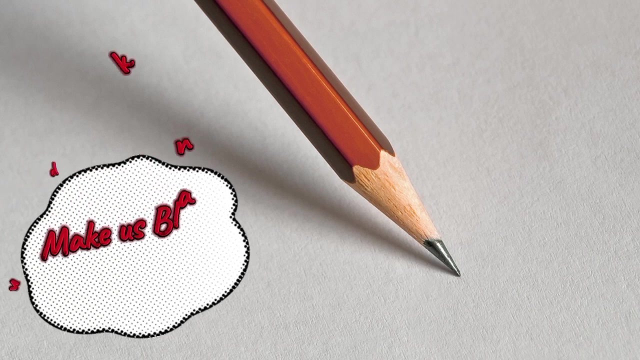 So we have a very weird tendency of cheating a lot of the way with this, like sleeping all air and nothing. So let's get to the topic, that is, multiple choice questions and how you can pass them. As you know, the exam setters have the mind that they have to set all confusing questions in order to confuse the students and make them blank. 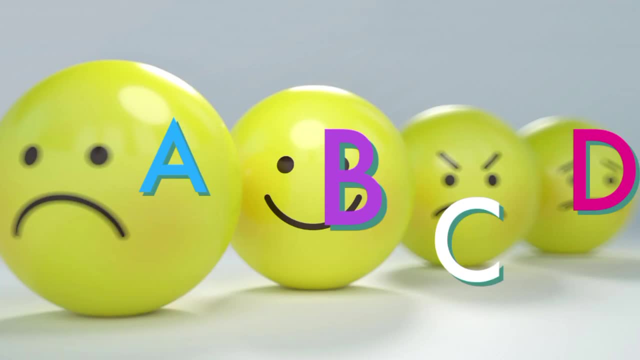 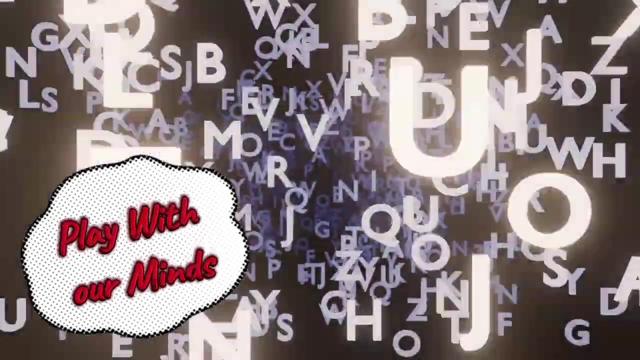 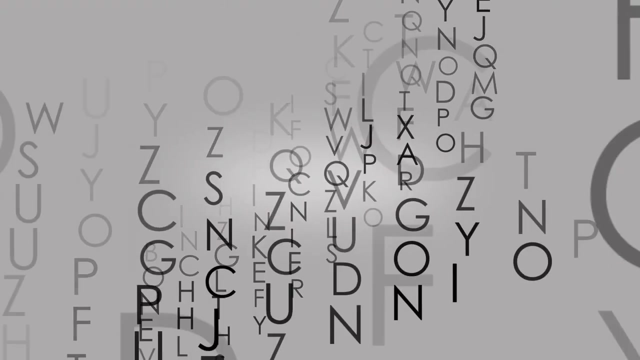 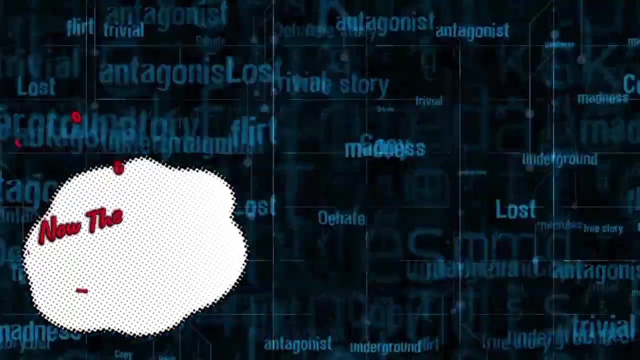 They give options A, P, C, D in the bubble sheets And while you're quite confused that which one is the right answer, You're entered into the world of confusion right after the paper is in your hand. Well, it is a very common thing that the bank effect that has been affected by many of the people. 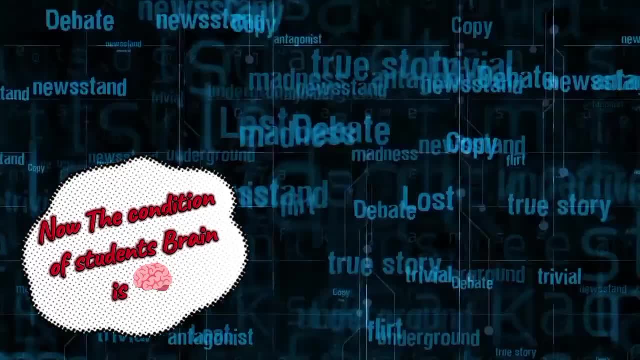 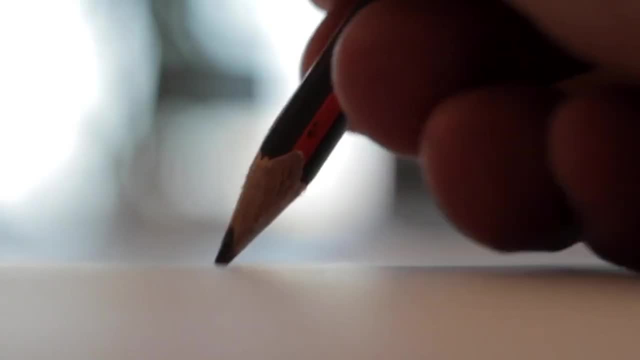 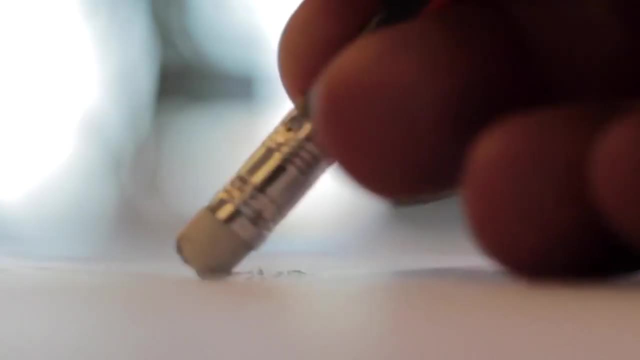 A lot of things scattered in our mind, that which one is the right answer, Which answer is right. These things continuously hitting our mind. So keep in mind, first of all, while you are writing, focus. Focus is an important thing that you must keep in your mind to not panic. 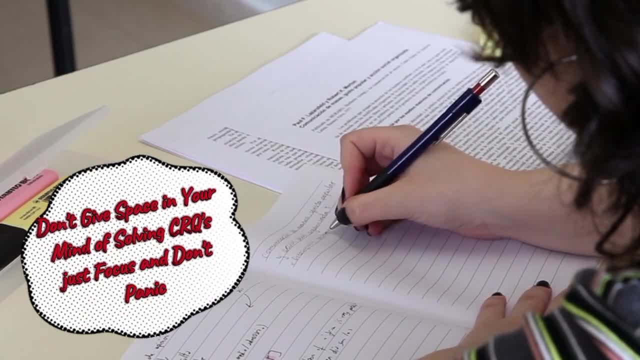 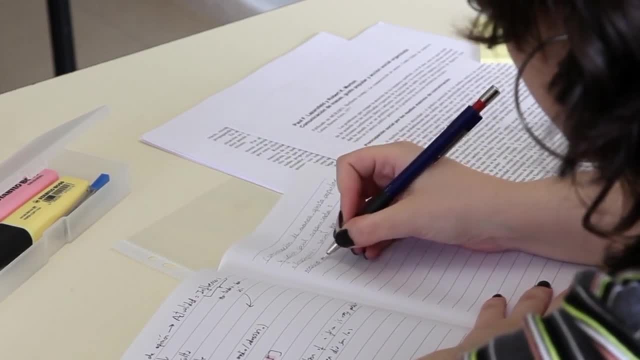 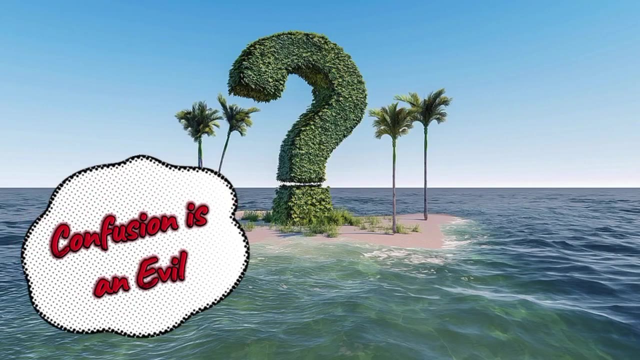 First thing. Secondly, to not keep your focus on long questions. on the subjective part, just focus on short questions and one thing in mind: Well, at the MCQs, have a deep relationship with your seductive portion. So still confused that how to solve these MCQs. 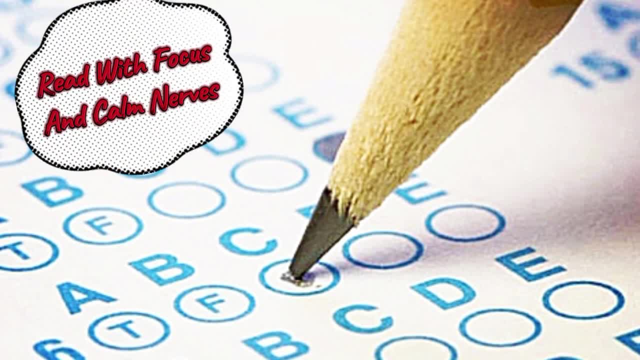 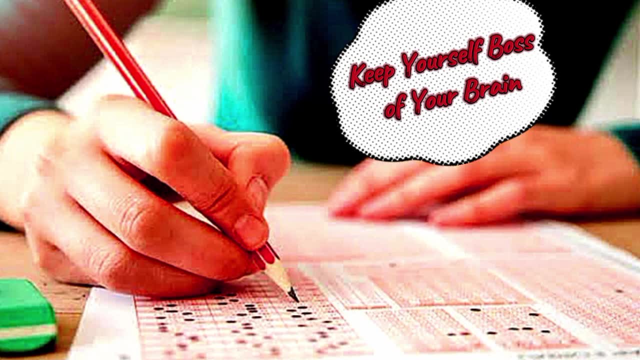 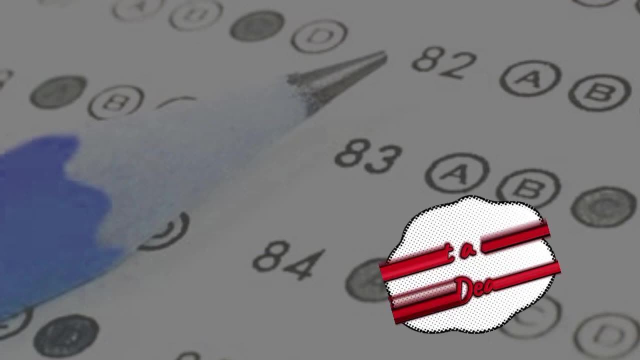 A lot of questions in our mind, Whether it is A, it is P, it is C or T, So there is nothing to worry about it. I'm going to tell you a brilliant method, And which you can easily understand, that how. 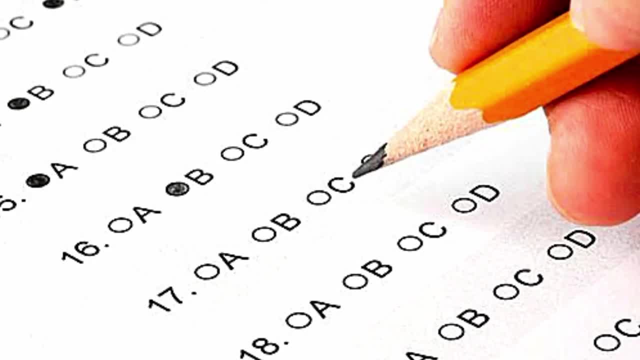 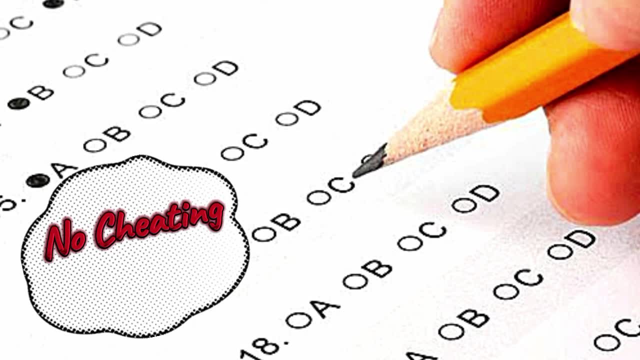 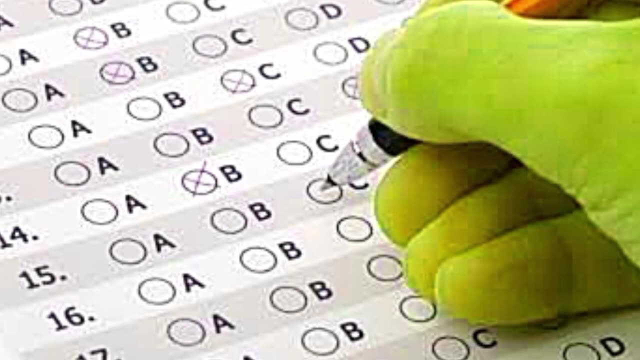 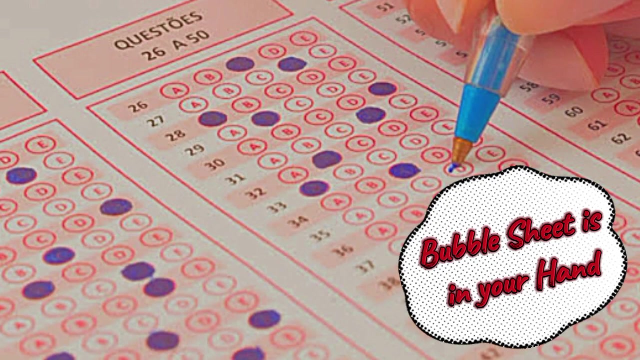 You can at least, without cheating and any other thing, get easily past that examination, all sort of examination, either with your school board exam or anything. right now you have in this form of bubble sheet in front of you. First thing you will have to do is to calm your nerves and to write the paper in different portions. 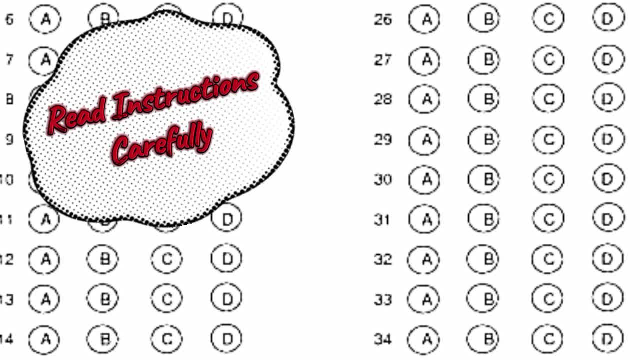 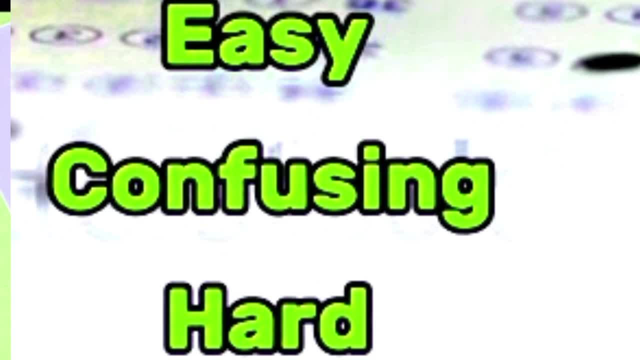 These things Are just in front of you. Then to see this bubble sheet. Let's confuse number one tip. Always remember number P option is more than 90% right. Write the paper in three parts: Easy, confusing and hard questions. 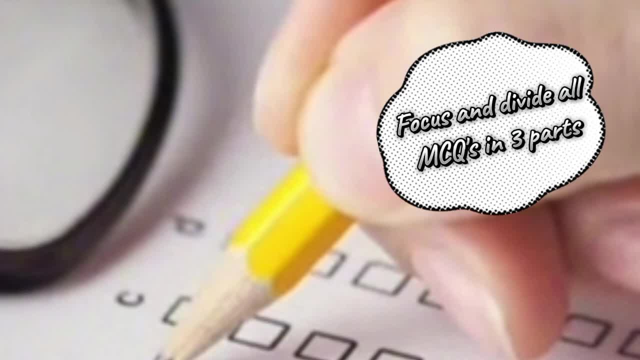 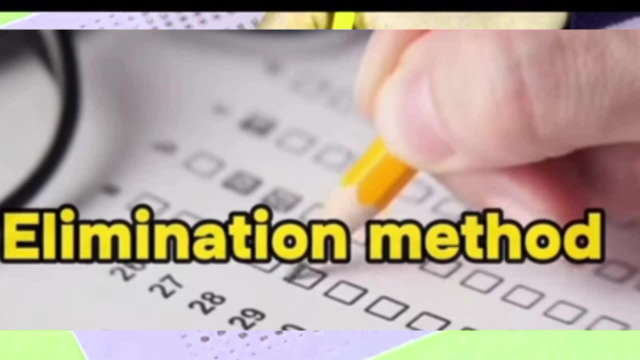 So let's start When you're writing To do ask your paper and questions in three parts. Number one thing: Elimination method. There are four options. You can eliminate two Types of questions. You have three types of questions. 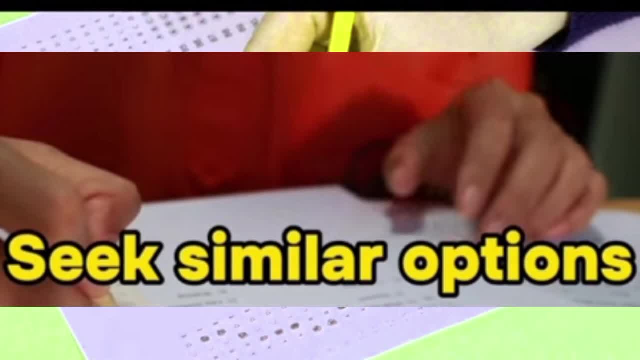 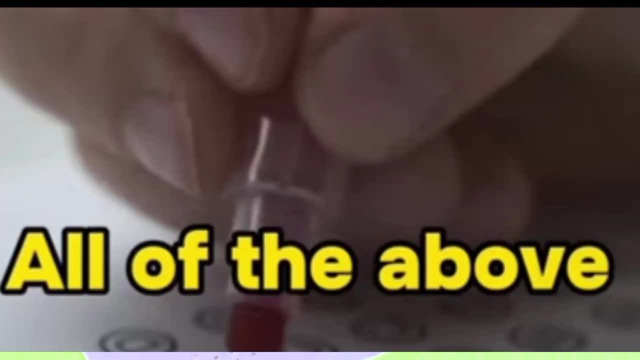 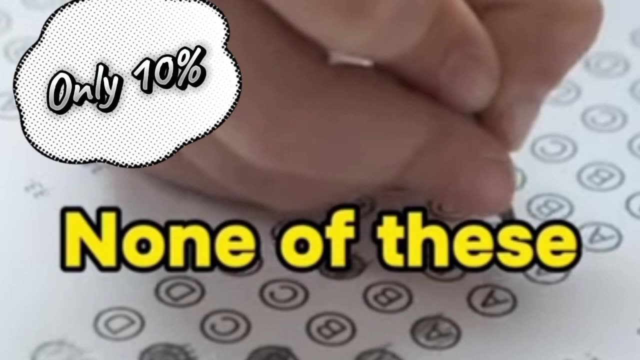 Easy, confusing and hard. Similar, Seek similar options Which are similar, ABCD. Eliminate them And just focus on the remaining. When you have questions, all of the above, Mostly 10%, these are right- And when none of these is returning the option. 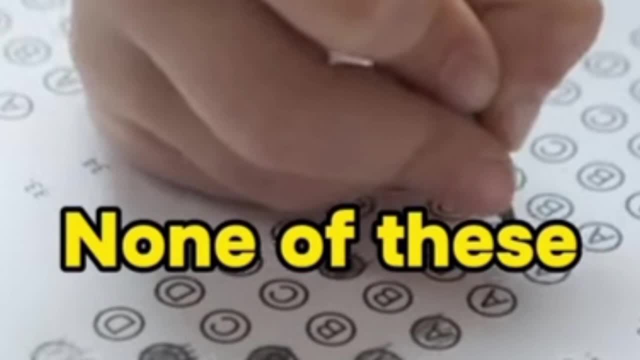 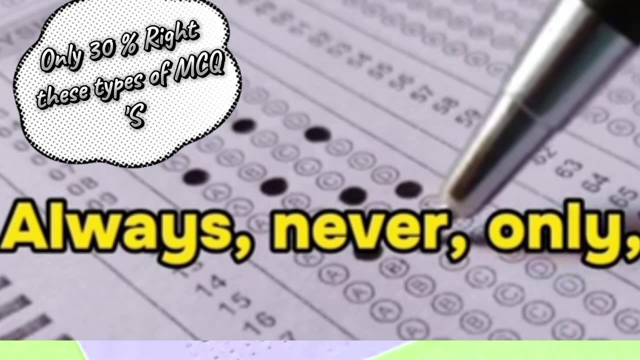 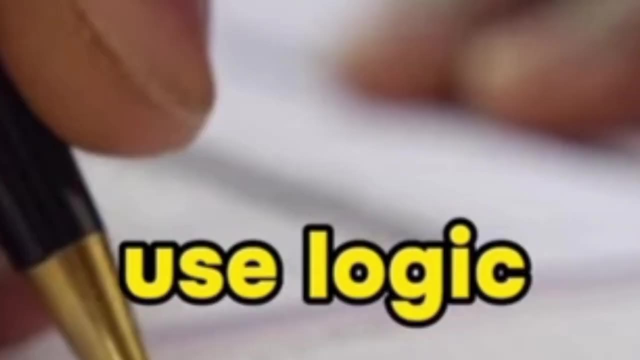 Mostly 30%. None of these option is a right. Always, never, only have extreme terms, Always ignore them. They're always wrong. Middle option is more than 90% that your middle option is right. Use logic. Think of a question. 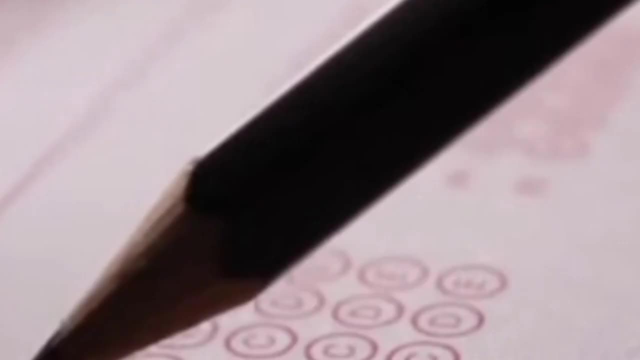 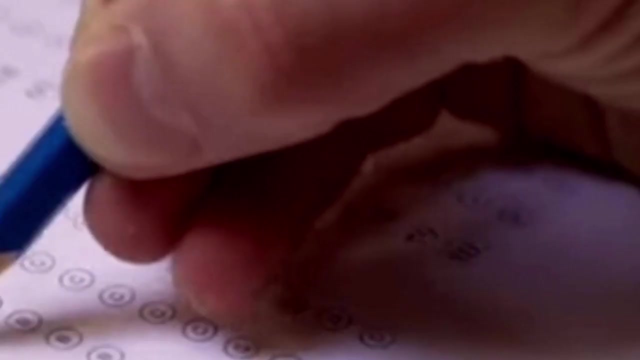 And think of practical application, You'll soon find a gate to that option. Don't panic, Don't hesitate And don't be so fast. Just focus On time And use logical answers. only Lot of examples I can tip on you. 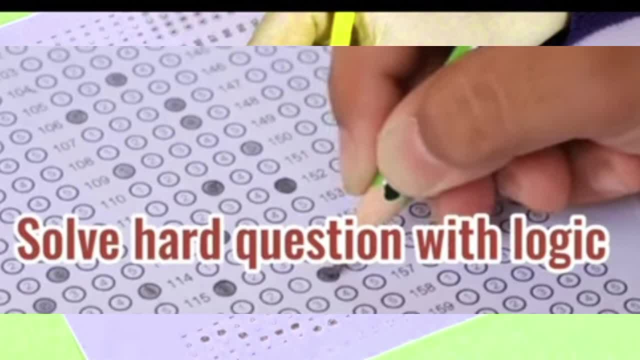 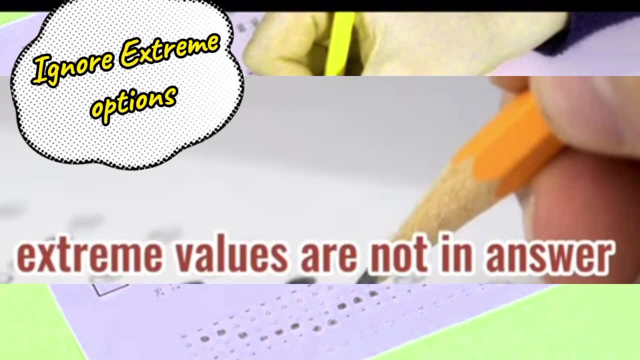 Now Solve hard questions with logic. When you are solving the hard questions, Just use your logical and IQ well. Extreme values are not in answers. When we have different options And there is some option that type extreme value, Ignore that answer.